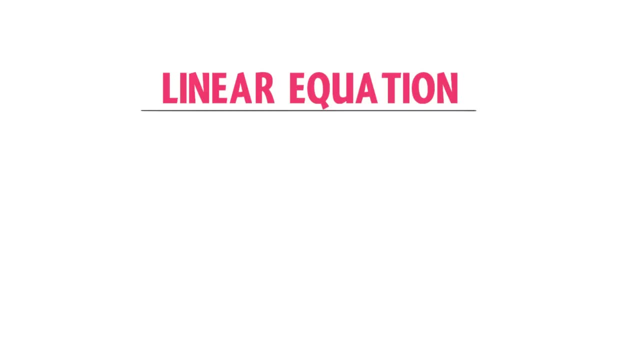 Linear equation. In this lecture, we will discuss about linear equation in one variable and linear equation in two variables or first degree equations. If I write 4x plus y is equal to 6. In this equation, there are three terms, 4x, y and 6. The x and y are known as variables, while 6 is the constant and 4 is the coefficient of variable x. The highest 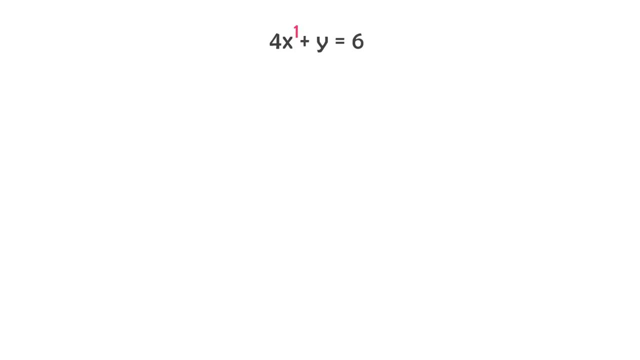 power of the variable x is 1 and the highest power of the variable y is also 1. Hence, all the variables in this equation have the highest power 1. Therefore, this equation is known 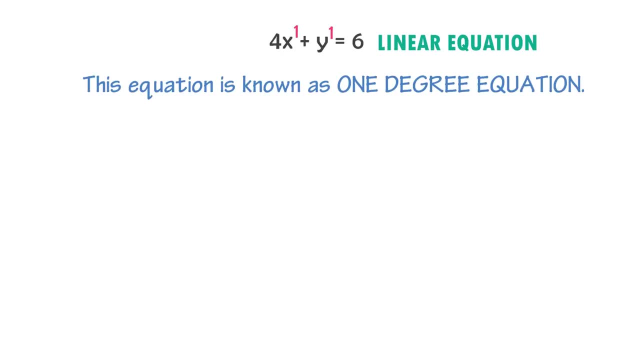 as a one degree equation or linear equation. Let me give you another example. 2xy plus 5 is equal to 10. This equation has also three terms, 2xy, 5 and 10. The term 2xy is considered as a one term. The power of x is 1, and the power of y is also 1. Hence, 1 plus 1 is equal 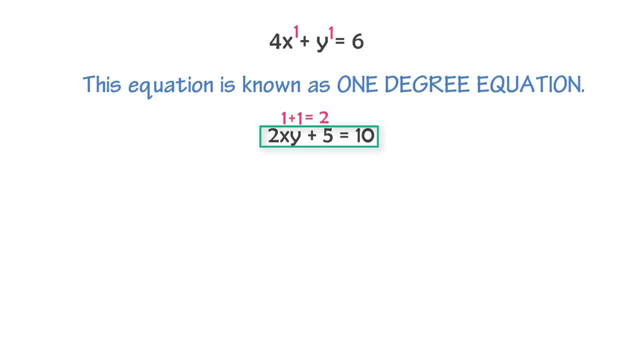 to 2. Thus the highest power of this equation is 2.therefore it is not one degree equation. 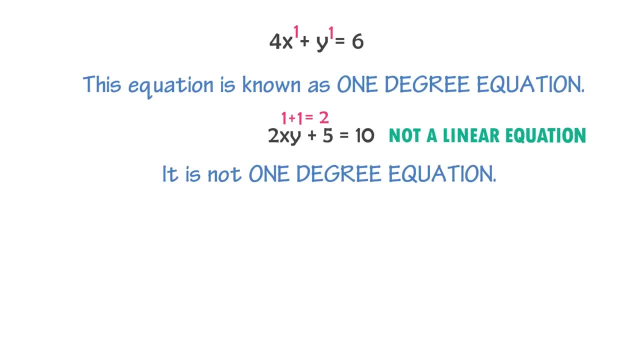 Hence it is also a linear equation. Now again if I write 3x plus 4yz plus xz is equal to 80. In this equation, we have 3x plus xz plus网C menos 0n. Which means this conditions is 2s, 30, 40, 60, 35 and a little less than 60 degrees. Now again if I write 3x plus Mommyz plus daily 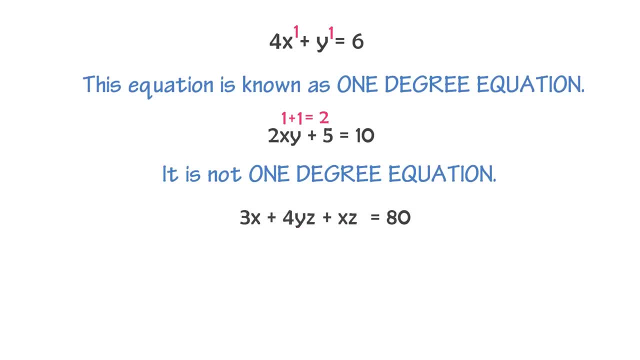 In this equation, there are four terms, the power of first term x is 1, the power of second term y is 1 and the power of z is also 1, hence 1 plus 1 is equal to 2, thus the power of second term is 2. 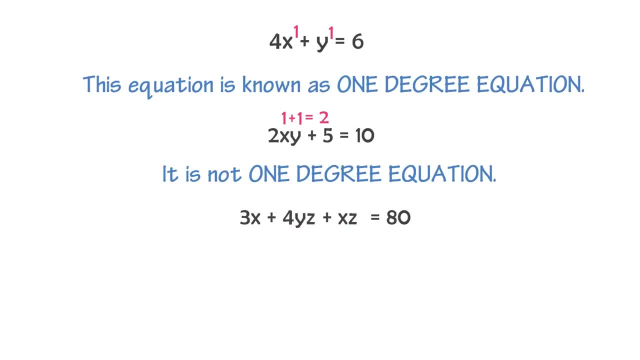 Four degrees, as in the other equation, a connect dimension of a value arrangement. each. there are four terms: The power of first term, x, is 1.. The power of second term, y, is 1.. And the power of z is also 1.. Hence 1 plus 1 is equal to 2.. Thus, the power of second term. 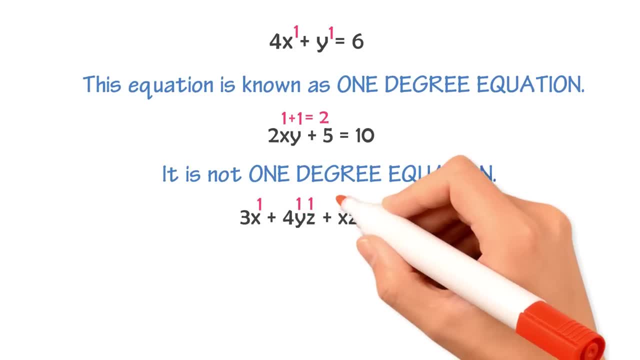 is 2.. The power of third term, x, is 1. And the power of z is also 1.. Hence 1 plus 1 is equal to 2.. Thus the power of third term is also 2.. So we can say that the highest power 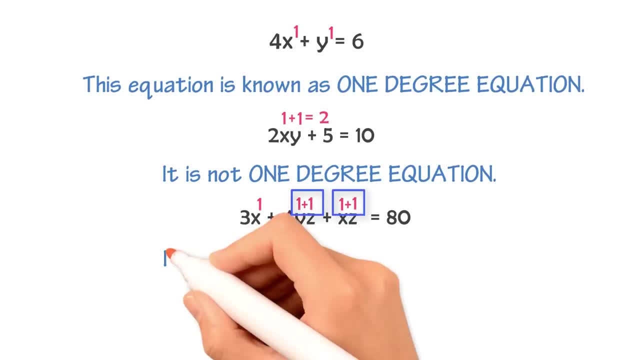 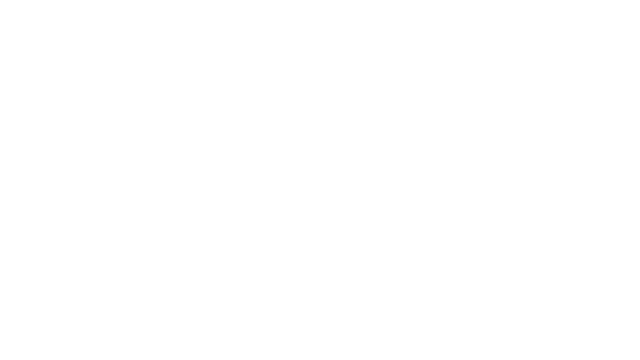 of this equation is 2.. Hence it is neither one degree equation nor linear equation. Similarly, if I write 2i plus 4 upon x is equal to 10.. Can you guess the highest power of this equation? Let me calculate it for you. 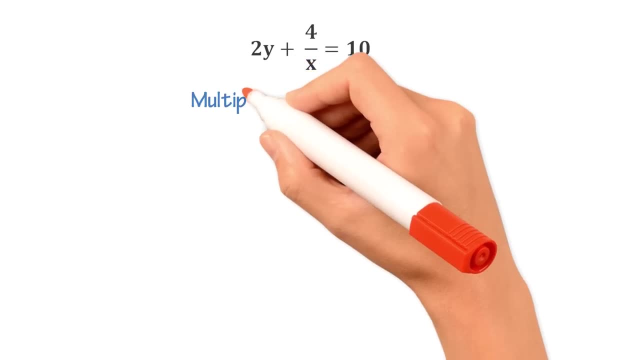 To simplify this equation: we multiply both sides by x. We get x into 2i plus x. 4 upon x is equal to 10x. Here x and x are cancelled out. As a result, we get 2xy plus 4 is equal. 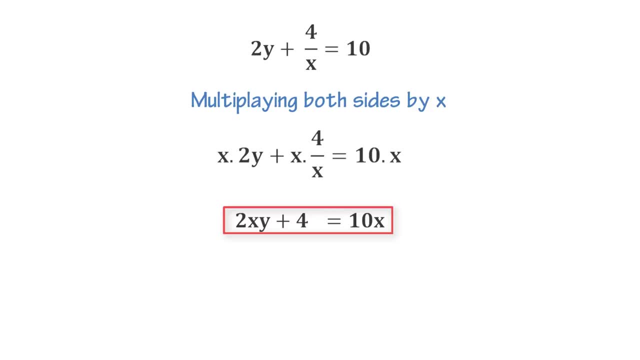 to 10x. Now there are three terms in this equation: The two variables and first term. 2xy is evaluated as follow: The power of x is 1. And the power of y is also 1.. Thus 1 plus 1 is equal to 2.. Hence the highest power of first term is: 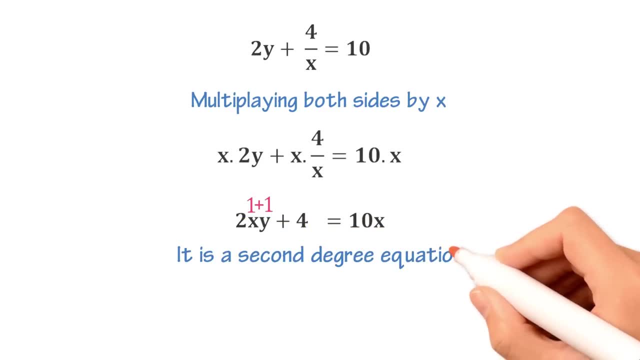 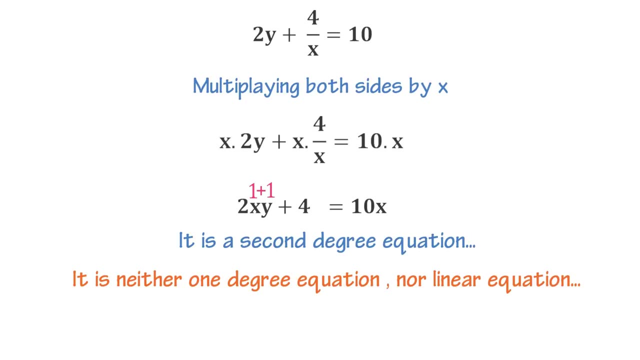 2. So it is a second degree equation. Therefore, it is neither one degree equation nor linear equation. Now let me give you one last example. 3a plus 4b plus 7c is equal to add d. Can you guess its highest power? I hope so. 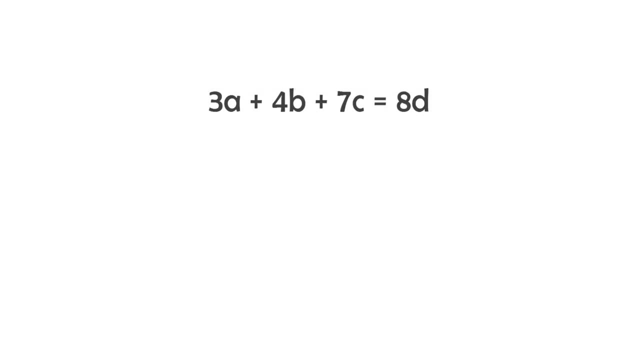 There are four terms in this equation. The power of a is 1., The power of b is 1.. The power of c is 1.. And the power of d is also 1.. Hence, the highest degree of this equation is 1.. Thus, 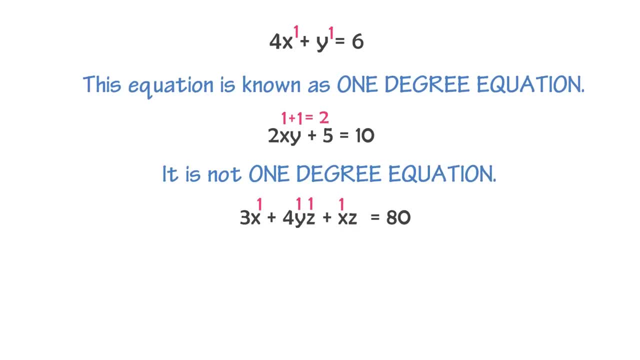 The power of third term x is 1 and the power of z is also 1, hence 1 plus 1 is equal to 2, thus the power of third term is also 2, so we can say that the highest power of this equation is 2, hence it is neither one degree equation nor linear equation. 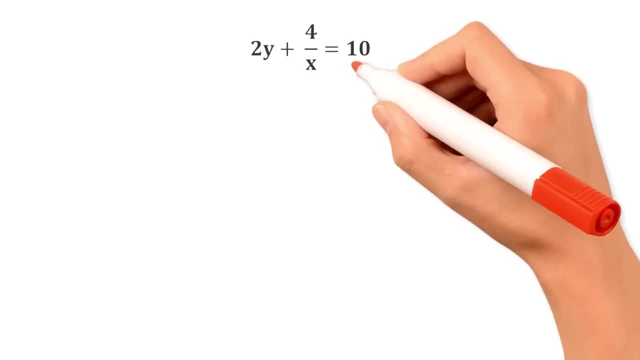 Similarly, if I write 2i plus 4 upon x is equal to 10, can you guess the highest power of this equation? Let me calculate it for you. 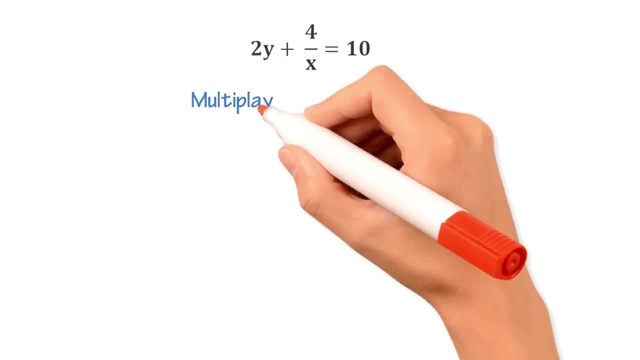 To simplify this equation, we multiply both sides by x, we get x into 2i plus x 4 upon x is equal to 10x, here x and x are cancelled out, as a result we get 2xy plus 4 is equal to 10x. 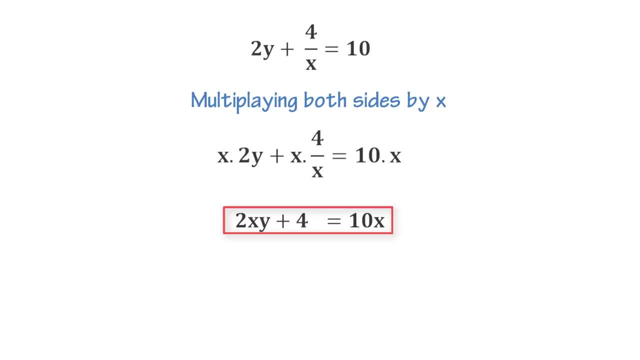 Now, there are three terms in this equation. The power of variables is 1. In the first and second terms, 2xy is evaluated as follows. 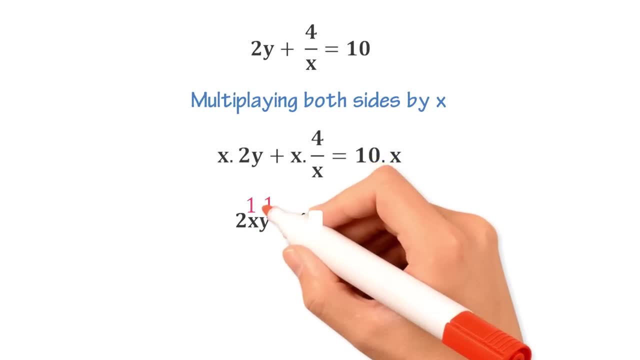 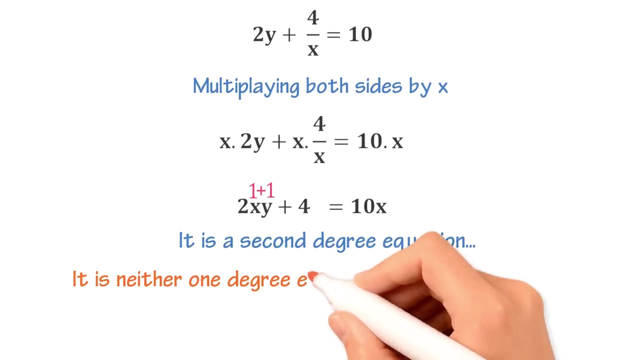 The power of x is 1 and the power of y is also 1, thus 1 plus 1 is equal to 2, hence the highest power of first term is 2, so it is a second degree equation, therefore it is neither one degree equation nor linear equation. 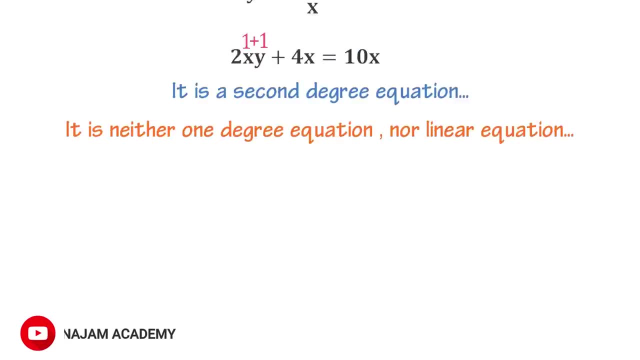 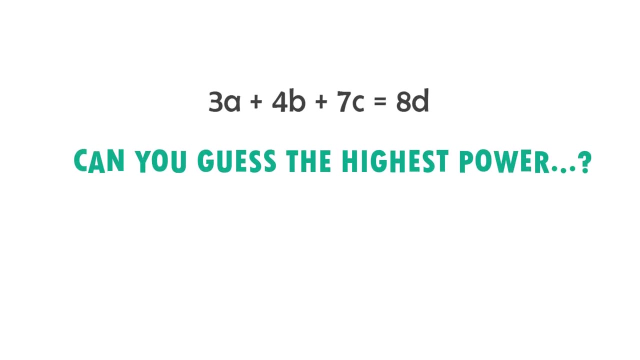 Now, let me give you one last example. 3a plus 4b plus 7c is equal to add d. Can you guess its highest power? I hope so. There are four terms in this equation. 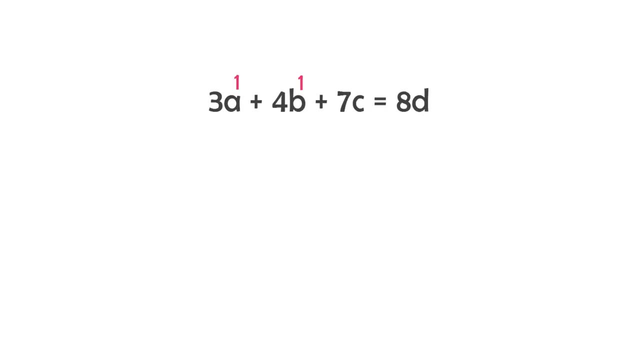 The power of a is 1, the power of b is 1, the power of c is 1 and the power of d is also 1, hence the highest degree of this equation is 1. 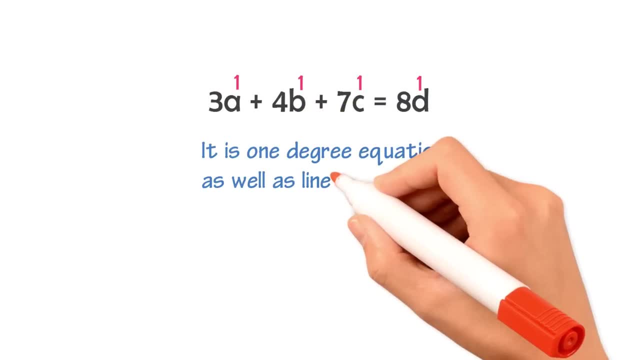 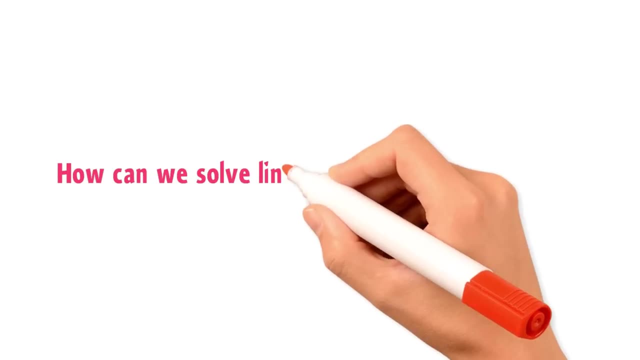 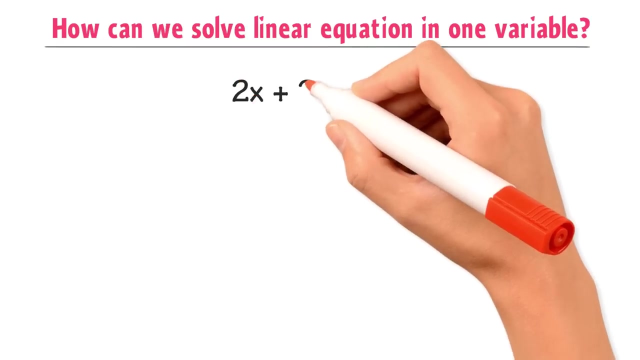 Thus, it is one degree equation. Now, let me teach you that how can we solve linear equation and one variable. For example, if a linear equation 2x plus 20 is equal to 50 is given and we are asked 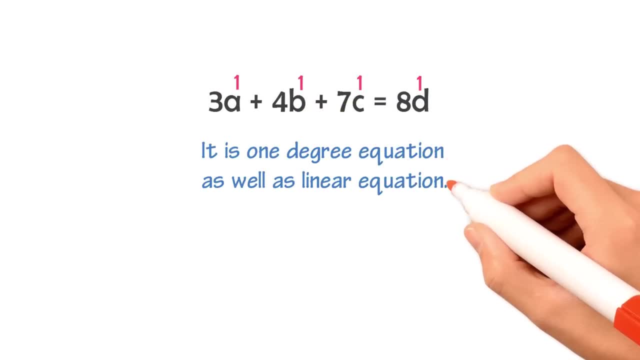 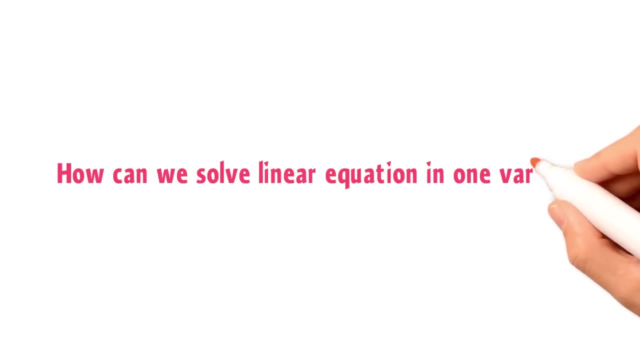 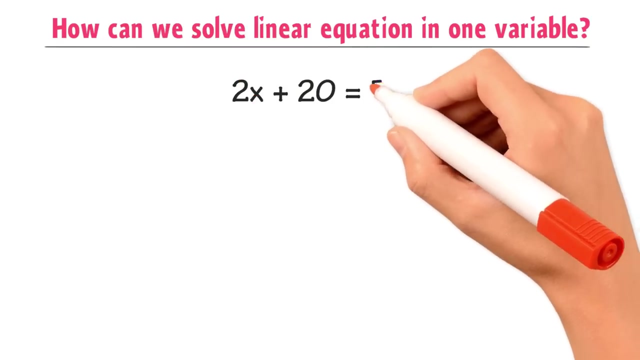 it is one degree equation. Now let me teach you that how can we solve linear equation and one variable? For example, if a linear equation- 2x plus 20 is equal to 50- is given and we are asked to find the value of x, Then it will be calculated as follow. Remember that this side of the equality sign. 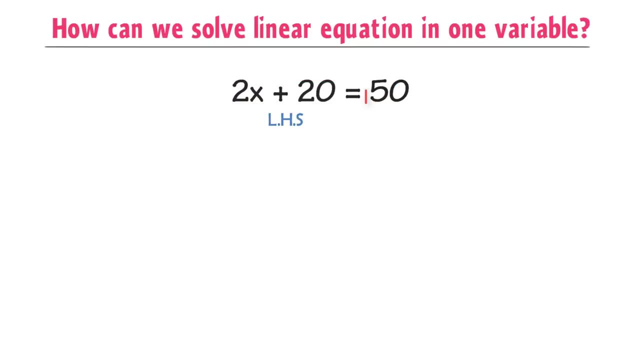 is known as a linear equation. So we have to find the value of x, Then it will be calculated as follow. Remember that this side of the equality sign is known as a linear equation. Do the same with the left hand side, While this side of the equality sign is known as: 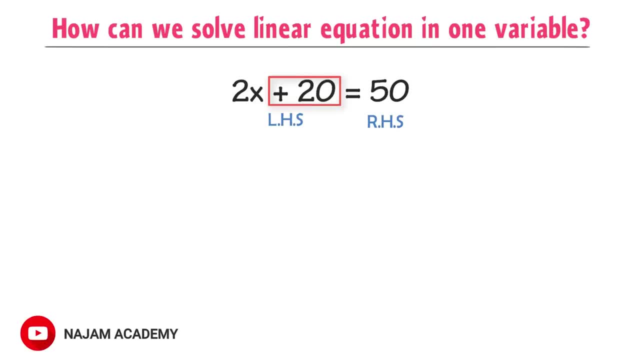 a right hand side, Now shifting plus 20 from the left hand side to the right hand side. As a result, the positive sign of 20 will be changed into negative sign. Hence, 2x is equal to 50 minus 20, or 2x is equal to 30. Now dividing both sides by 2.. So you can see. 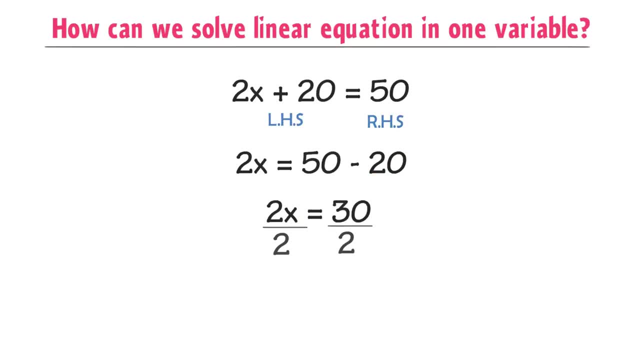 2x divided by 2 is equal to 30 divided by 2. as a result we get: x is equal to 15. now let me give you another example: 30 minus y is equal to 2y. we know that there are three terms in this equation, but there are two terms in which there 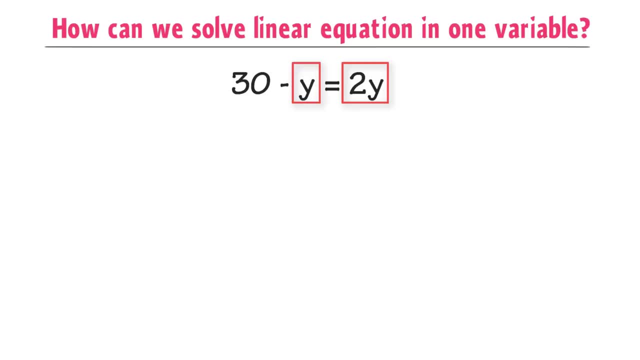 is the same variable. I mean y. hence we will arrange this equation in a way in which y should be made as a one term. thus we will shift minus y from the left-hand side to the right-hand side. as a result, we will get: 30 is equal to 2y. 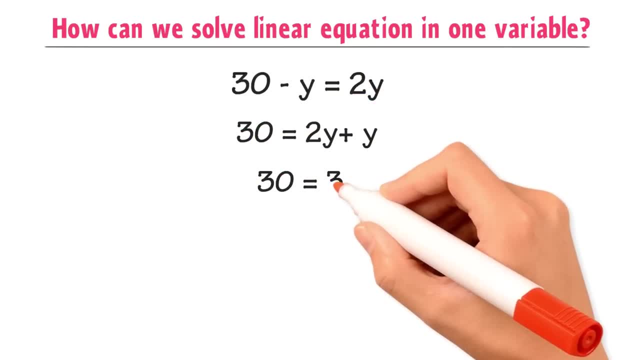 plus y, our 30 is equal to 3y. now, dividing both sides by 3, 30 divided by 3 is equal to 3y divided by 3. thus we get y is equal to 10. now let me teach you one advanced or multiple steps type of linear equation. 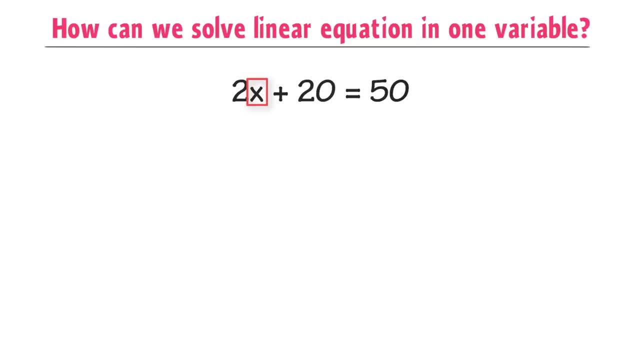 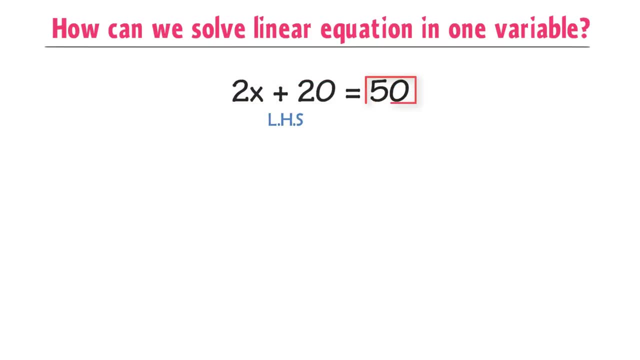 known as a left hand side. While this side of the equality sign is known as a right hand side. Now shifting plus 20 from the left hand side to the right hand side. As a result the positive sign of 20 will be changed into negative sign. Hence 2x is equal to 50 minus 20. Our 2x is equal 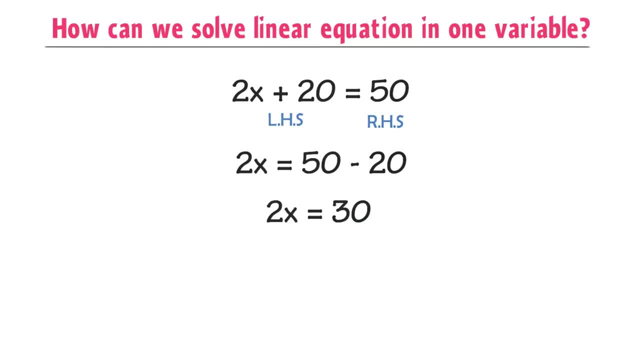 to 30. Now dividing both sides by 2. 2x divided by 2 is equal to 30 divided by 2. As a result we get x is equal to 15. Now let me give you another example. 30 minus y is equal to 2y. 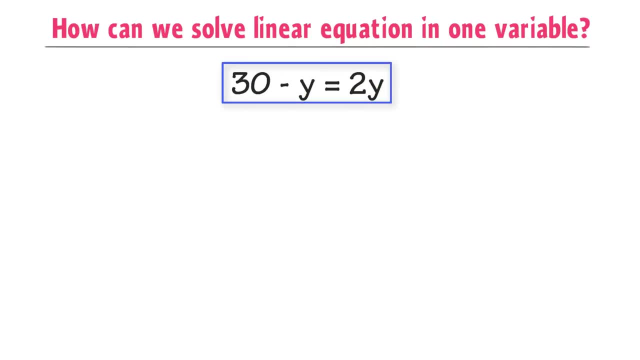 We know that there are three terms in this equation. But there are two terms in which there is the negative sign. Now let me give you another example. 30 minus y is equal to 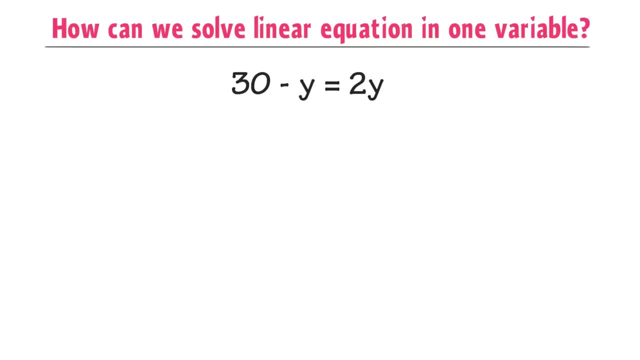 the same variable. I mean y. Hence we will arrange this equation in a way in which y should be made as a one term. Thus we will shift minus y from the left hand side to the right hand side. 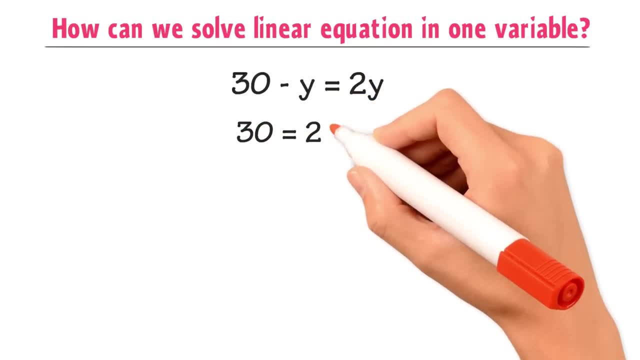 As a result we will get 30 is equal to 2y plus y. Our 30 is equal to 3y. Now dividing both sides by 3. We know that there are three terms in this equation. But there are two terms in this equation. Hence we will shift minus y from the left hand side to the right hand side. Thus we will shift minus y from the left hand side to the right hand side. Hence we will shift minus y from the left hand side to the right hand side. 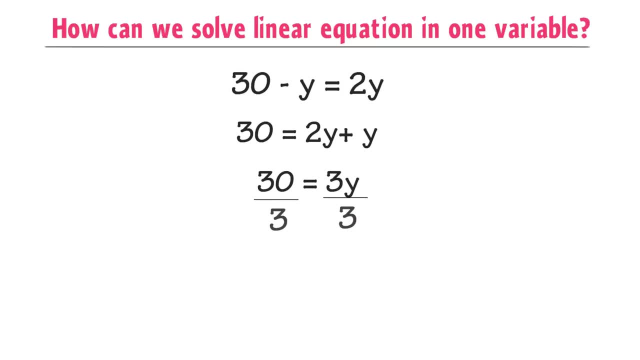 30 divided by 3 is equal to 3y divided by 3. Thus we get y is equal to 10. Now let me teach you one 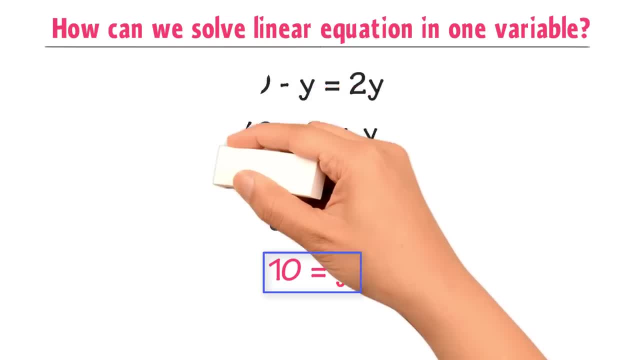 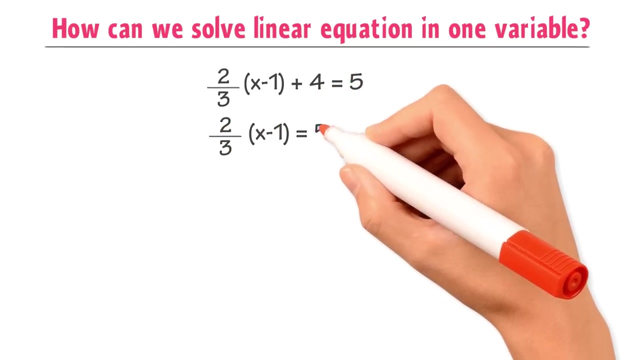 advanced or multiple steps type of linear equation and one variable. 2 upon 3 and to x minus 1 plus 4 is equal to 5. And this type of linear equation first of all shift the constant to one side. And variables to another side. Thus we are going to shift plus 4 from the left hand side to the right hand side. So 2 upon 3 x minus 1 is equal to 5 minus 4. Our 2 upon 3 and to x minus 1 is equal to 1. 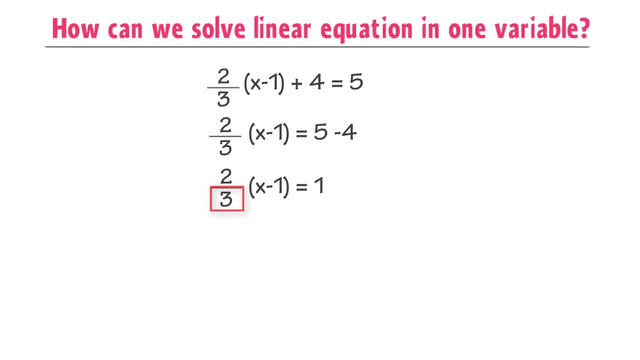 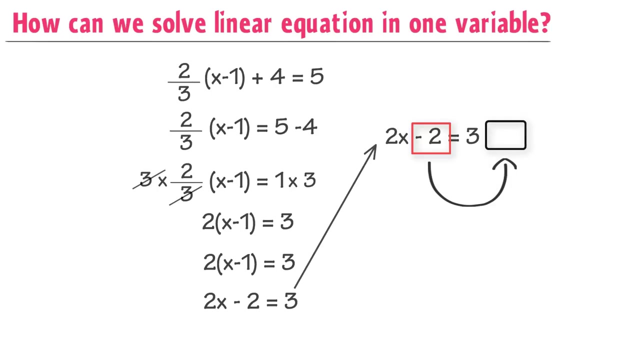 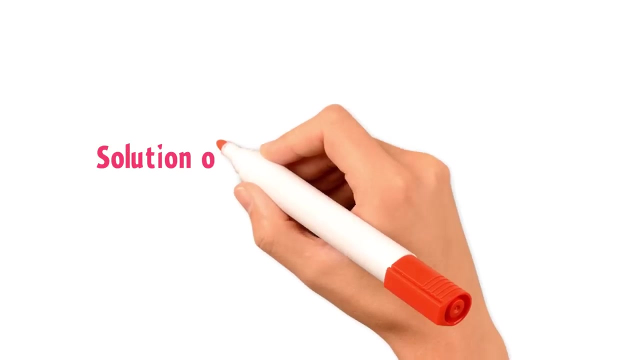 Now it is time to terminate 3 as a denominator. To do so we multiply both sides by 3. So we will write down 1 upon 2 which is 3 x minus 1 plus 3. 3 into 2 divided by 3 into x minus 1 is equal to 1 times 3. That is 1 and 3 is cancelled out. As a result, we get 2 and 2 x minus 1 is equal to 3. Or 2 x minus 2 is equal to 3. Now again we will shift minus 2 from the left hand side to the right hand side. Thus we get 2 x minus 1 x minus 1 plus 3. So the equal to 3 plus 2. Our 2x is equal to 5. So dividing both sides by 2. 2x divided by 2 is equal to 5 divided by 2. 2 and 2 are again cancelled out. As a result, we get x is equal to 5 divided by 2. Now let me teach you the solution of linear equation and two variables. 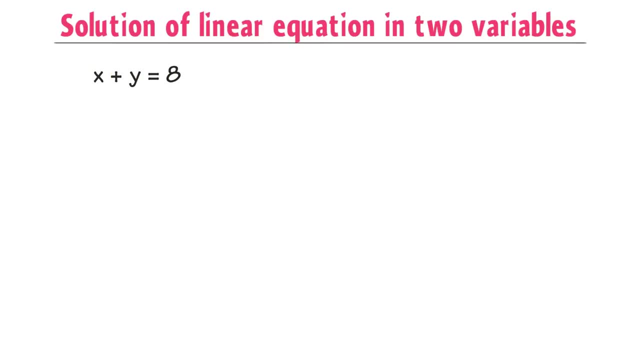 For example, x plus y is equal to add and x minus y is equal to 6. Let me call this equation number 1 and I call this equation number 2. Now, there are different methods of solving such type of linear equation. But I am going to solve this problem through a basic way. 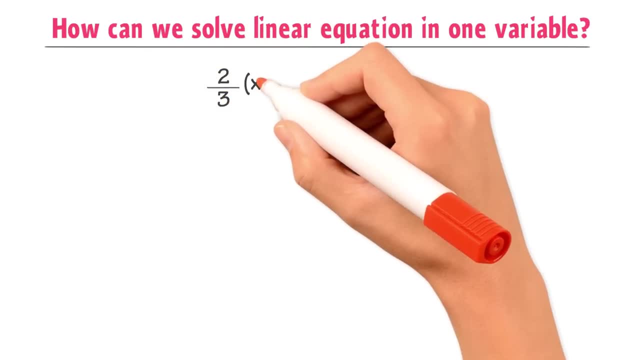 and one variable, 2 upon 3, and 2x minus 1 plus 4 is equal to 5. and this type of linear equation first of all shift the constant to 1 side and variables to another side. thus we are going to shift plus 4 from. 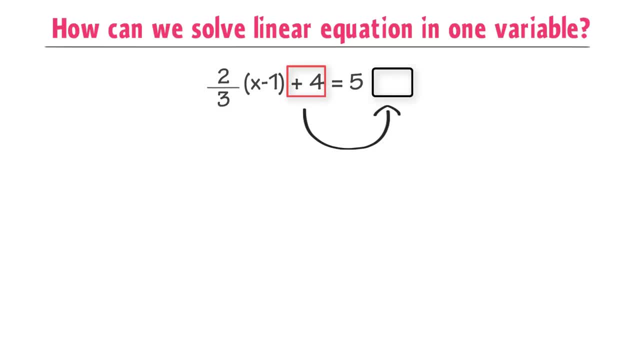 the left-hand side to the right-hand side. so 2 upon 3 x minus 1 is equal to 5 minus 4 are 2 upon 3, and 2x minus 1 is equal to 1. now it is time to terminate 3 as a denominator. to do so, we multiply by: 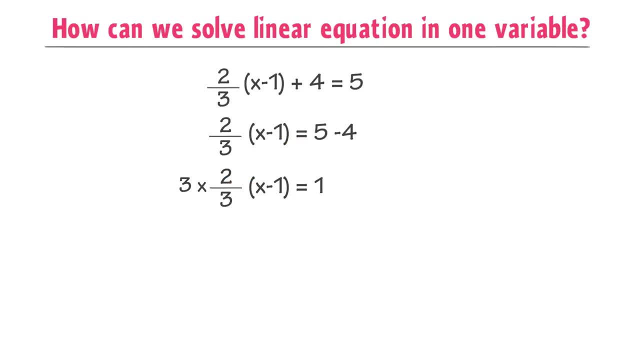 both sides by 3.. 3 into 2, divided by 3 into x minus 1 is equal to 1 times 3.. 3 and 3 is cancelled out. As a result, we get 2 into x minus 1 is equal to 3.. Our 2x minus 2 is: 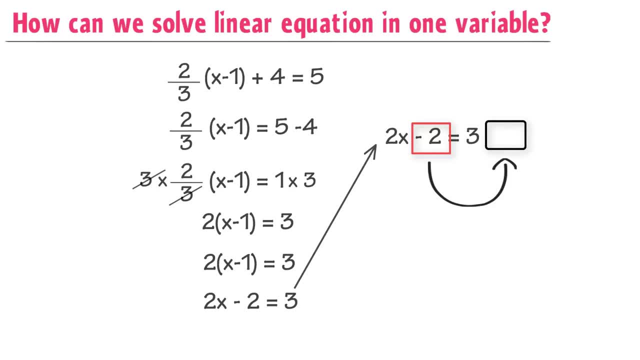 equal to 3.. Now again, we will shift minus 2 from the left hand side to the right hand side. Thus we get: 2x is equal to 3 plus 2. Our 2x is equal to 5. So dividing both sides. 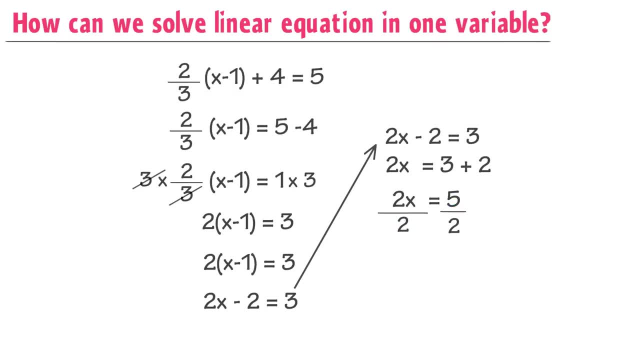 by 2.. 2x divided by 2 is equal to 5 divided by 2.. 2 and 2 are again cancelled out. As a result, we get: x is equal to 5 divided by 2.. Now let me teach you the solution of linear. 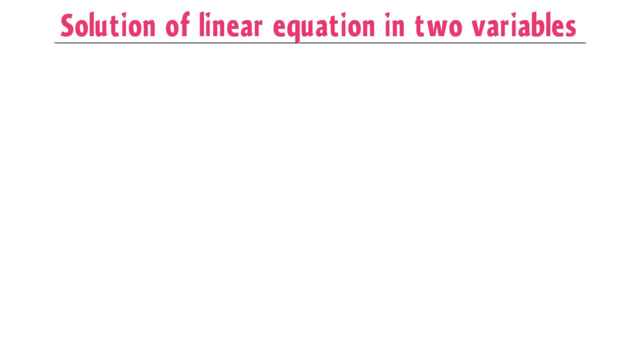 equation and two variables. For example, x plus y is equal to 8 and x minus y is equal to 6.. Let I call this equation number 1 and I call this equation number 2.. Now, there are different methods of solving such type of linear equation, But I am going to solve this problem through a basic way. 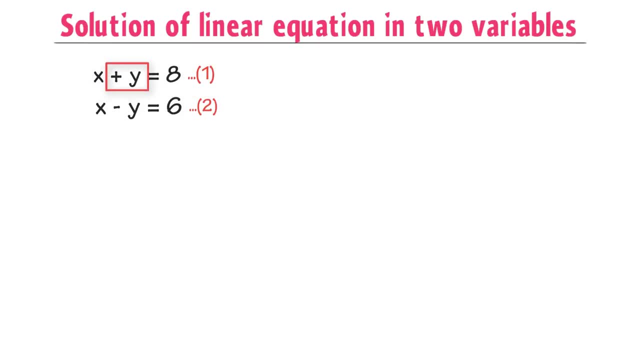 Now look at equation number 1, where the coefficient of y is plus 1.. Then look at equation number 2, where the coefficient of y is minus 1.. So if we add equation number 1 and equation number 2, plus y and minus y will be cancelled out And we will get only 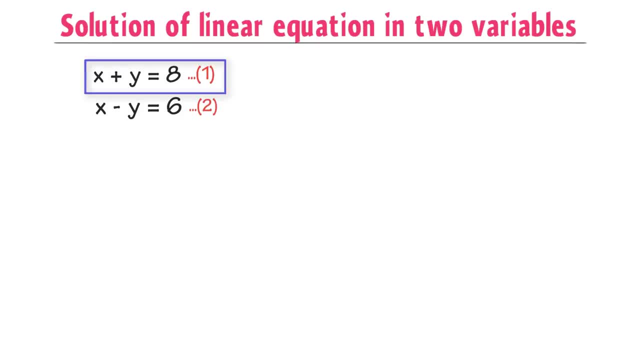 Now, look at equation number 1, where the coefficient of y is plus 1 and then look at at equation number 2 where the coefficient of y is minus 1. So if we add equation number 1 and equation number 2, plus y and minus y will be cancelled out and we will get only x variable and then solving one variable equation will be pretty easy job. Therefore adding equation number 1 and equation number 2, x plus y is equal to add plus x minus y is equal to 6. Here plus y and minus y are cancelled out. We get 2x is equal to 14. Now dividing both sides by 2, 2x divided by 2 is equal to 14 divided by 2. As a result we get x is equal to 7. So the final result is the following. 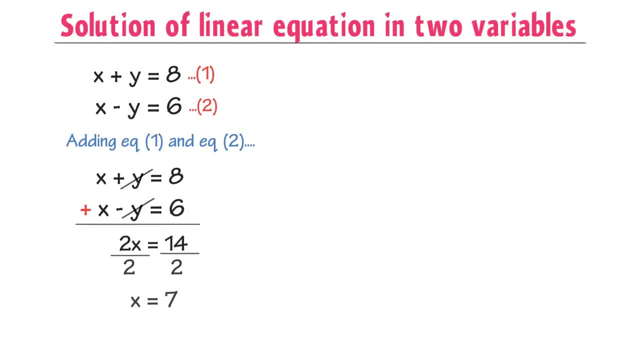 Now, what about the value of y? We can now easily calculate the value of y by substitution method by putting value of x in either equation number 1 or in equation number 2. Let me first put the value of x in equation number 1 and then in equation number 2. Now, equation number 1 is x plus y is equal to 8. We know that x is equal to 7. Thus, putting x is equal to 7 in equation number 1. 7 plus y is equal to 8. Now, shift plus 7 from the left-hand side to the right-hand side. 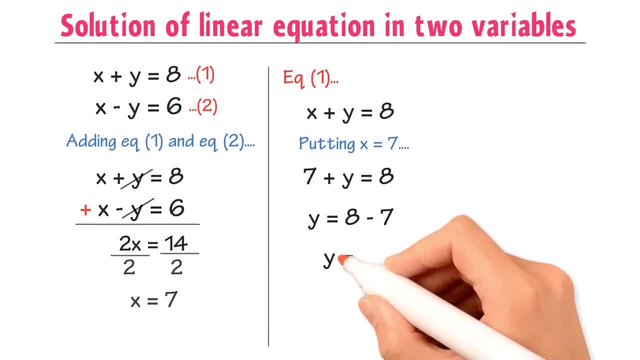 y is equal to 8 minus 7 or y is equal to 1. 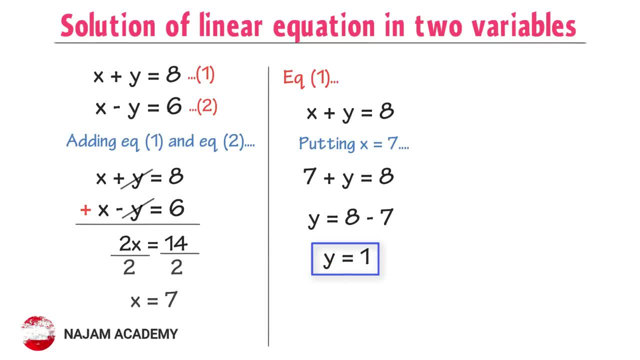 So, the value of y is 1 and the value of x is 7. 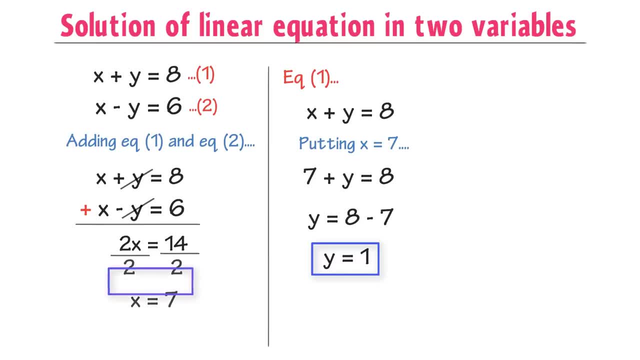 If you put the value of x in equation number 2, it will again give you the same value of y. Let me do it. We know that equation number 2 is x minus y is equal to 6 while the value of x is equal to 7. Hence, putting x is equal to 7 in equation number 2. 7 minus y is equal to 6. 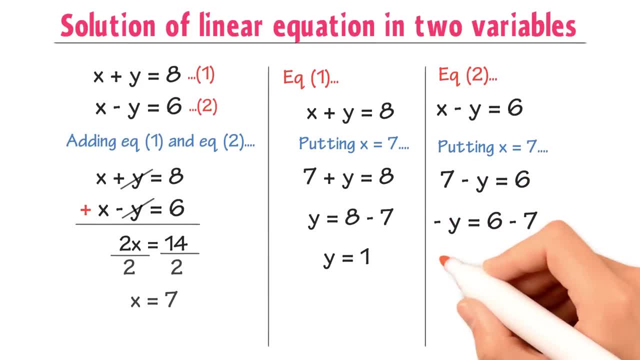 Now, minus y is equal to 6 minus 7 or minus y is equal to minus 1. Minus y is equal to minus 1. And minus sign are cancelled out. 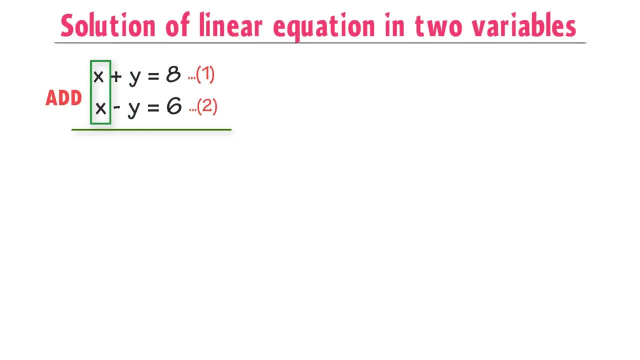 x variable And then solving one variable equation will be pretty easy job. Therefore, adding equation number 1 and equation number 2.. x plus y is equal to 8. equal to 8. plus x minus y is equal to 6.. Here plus y and minus y are cancelled out, We get 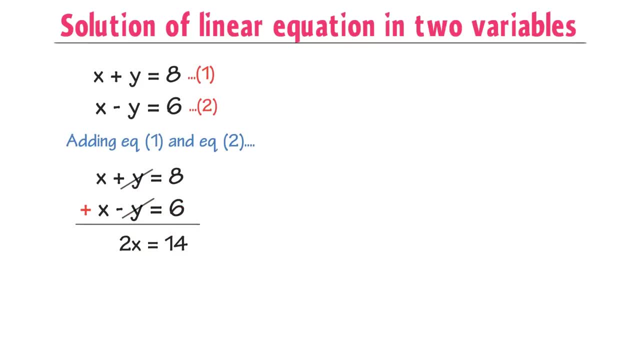 2x is equal to 14.. Now, dividing both side by 2,: 2x divided by 2 is equal to 14 divided by 2.. As a result we get: x is equal to 7.. Now, what about the value of y? We can now. 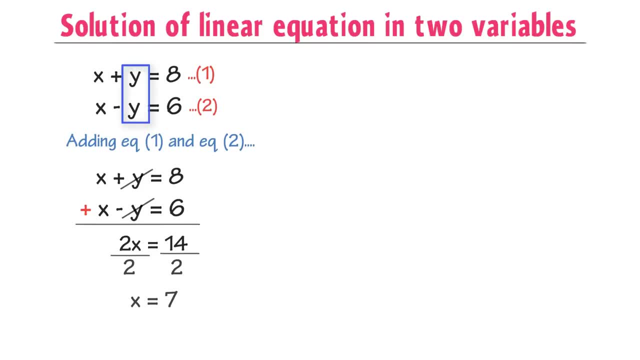 easily calculate the value of y by substitution method, by putting value of x in either equation number 1 or in equation number 2.. Let me first put the value of x in equation number 1 and then in equation number 2.. Now equation number 1 is x plus y is equal to 8. We know that. 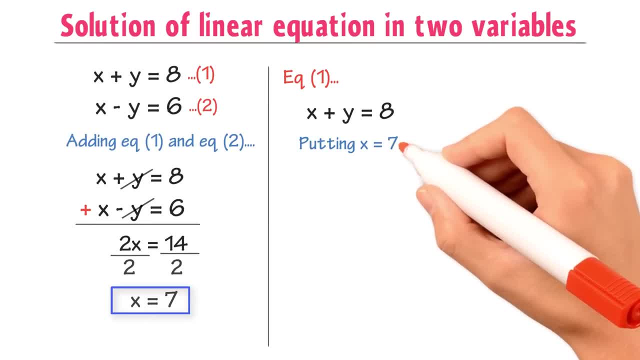 x is equal to 7.. Thus putting x is equal to 7 in equation number 1.. Now we can easily calculate the value of y by substitution method, by putting value of x in equation number 2.. 7 plus y is equal to 8.. Now shift plus 7 from the left hand. 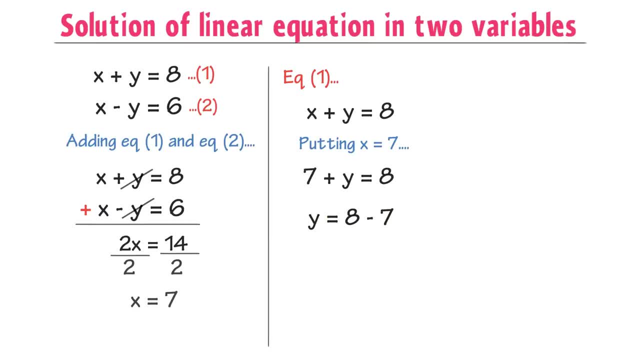 side to the right hand side, y is equal to 8 minus 7 or y is equal to 1.. So the value of y is 1 and the value of x is 7.. If you put the value of x in equation number 2, it: 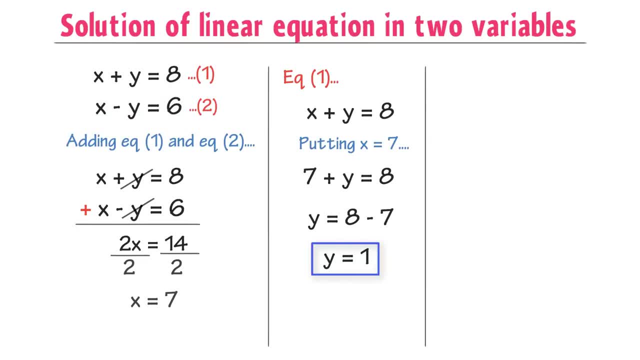 will again give you the same value of y. Let me do it. We know that equation number 2 is: x minus y is equal to 6, while the value of x is equal to 7.. Hence, putting x is equal to 7 in equation number 2.. 7 minus y is equal to 6.. Now minus. 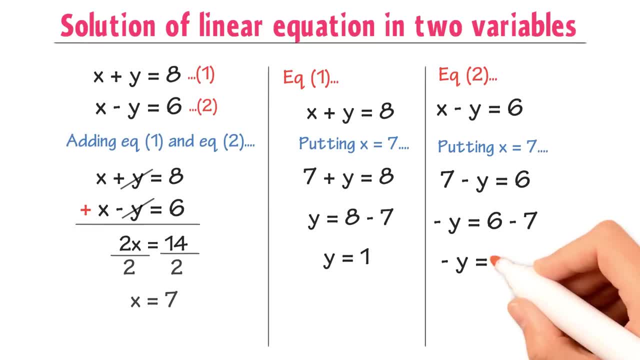 y is equal to 6 minus 7 or minus y is equal to minus 1.. Minus and minus sign are cancelled out. As a result, we get again: x minus y is equal to 6 minus 7 or minus y is equal to. 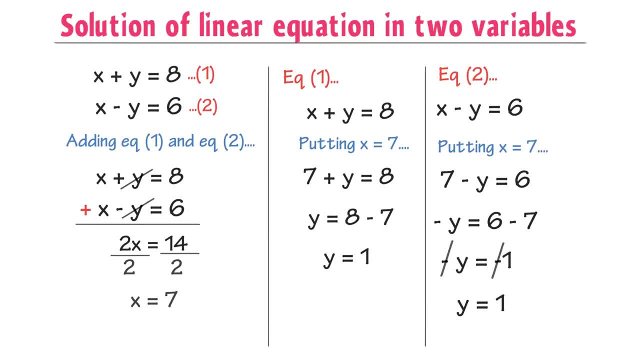 7. Again, y is equal to 1.. Thus we learn that either you put the value of x in equation number 1 or in equation number 2, it will always give you the same value of y.